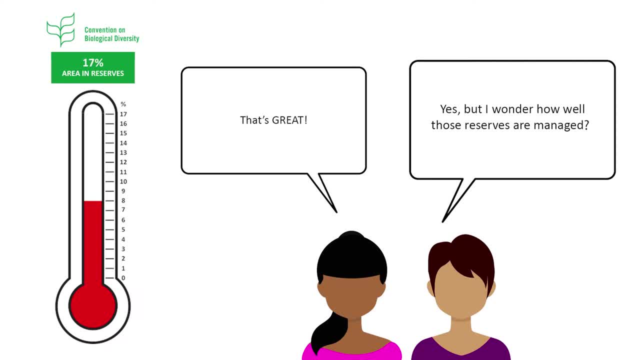 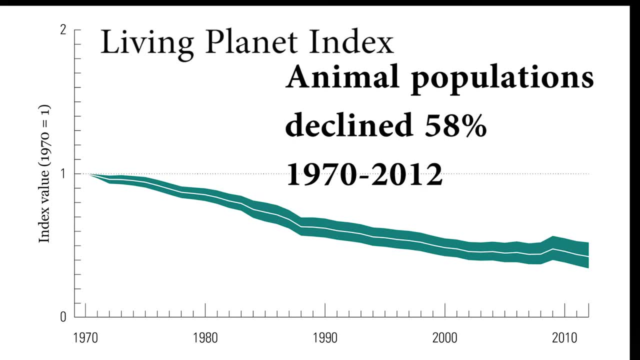 and the community what we need to achieve to save biodiversity, as well as measuring progress towards targets, But most of the indicators so far are showing that things are getting worse for biodiversity. The biodiversity crisis is escalating, despite nearly all nations agreeing to the targets. 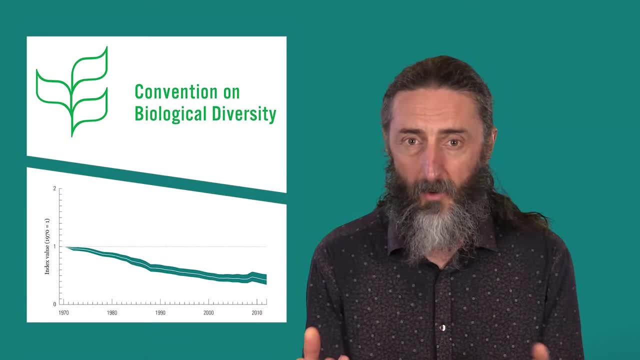 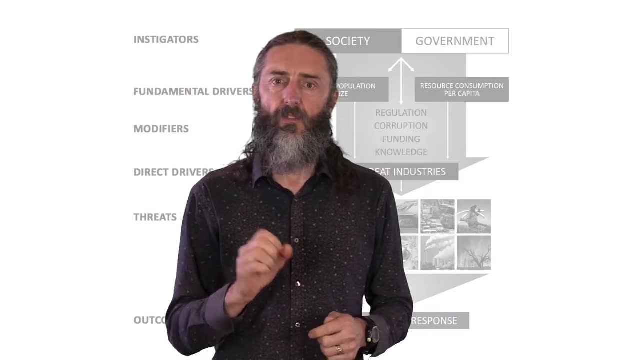 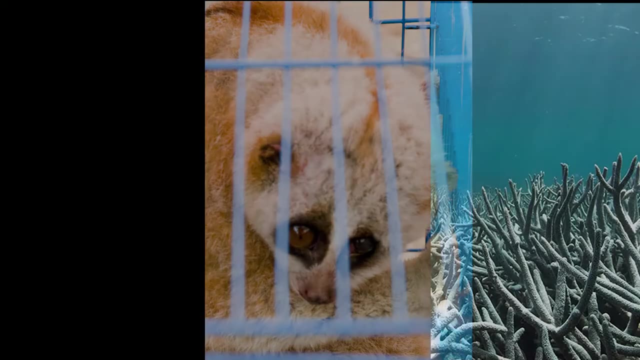 What is going wrong? What if we take a step out from what is being done and consider the full range of processes that drive biodiversity loss? So we have this disastrous loss of biodiversity, including loss of ecosystems, species extinctions and range contractions that erode genetic diversity, Directly causing this biodiversity. 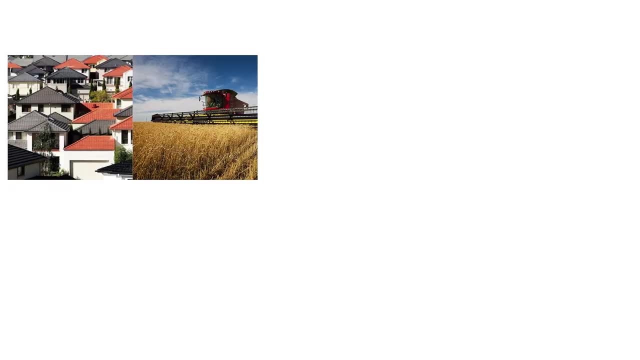 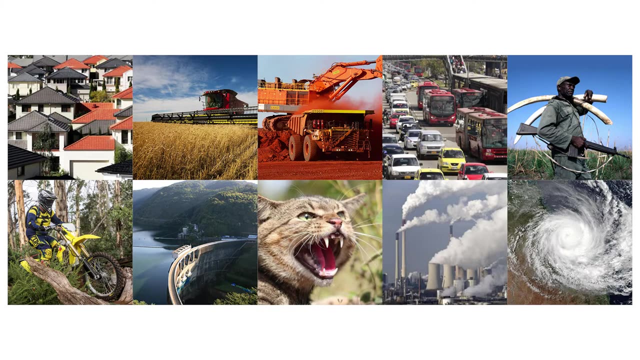 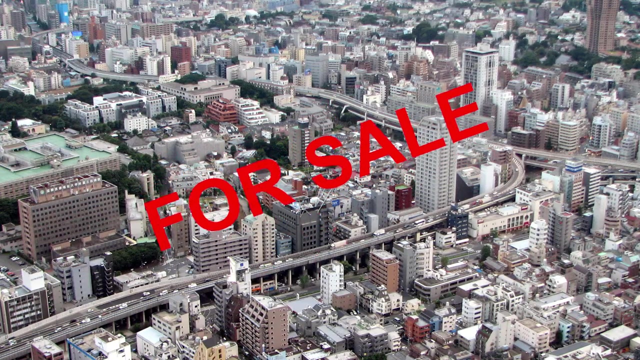 crisis are the direct threats – urbanisation, agriculture, mining, roads, hunting, recreation and war, dams and dams. And each of these immediate threats have direct drivers – the threat industries. For example, real estate developers are the direct driver of urbanisation, The pet, horticulture and 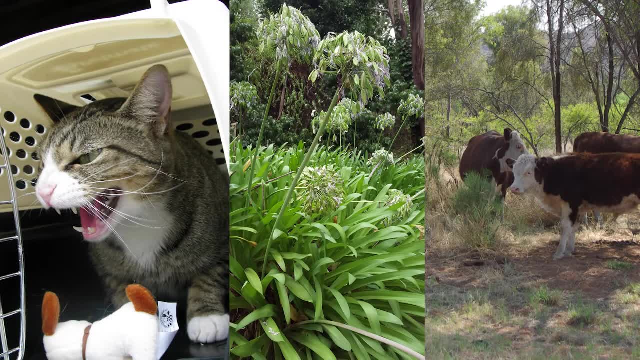 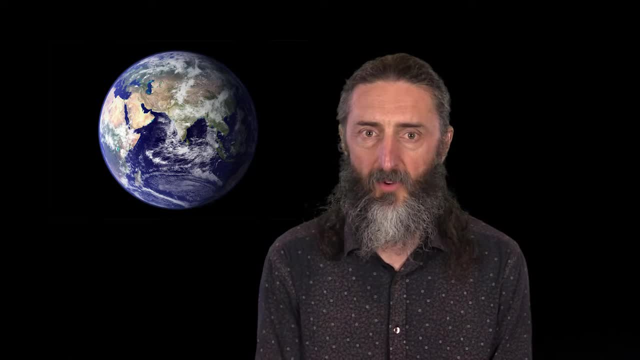 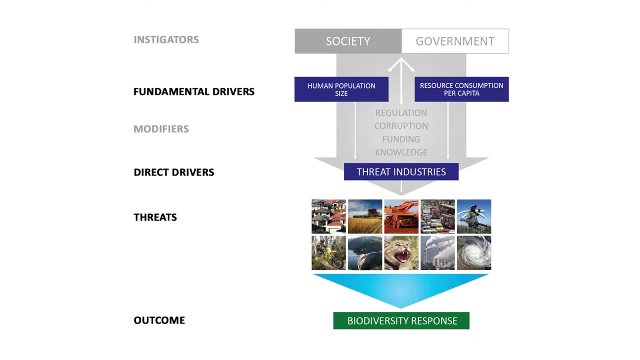 agriculture trades directly introduce and spread invasive species. These industries are in place to meet the increasing demands for resources by a growing human population. The number of people and how much each person consumes are the fundamental drivers of biodiversity loss. Right at the top of this hierarchy of drivers sit the instigators – society and government. 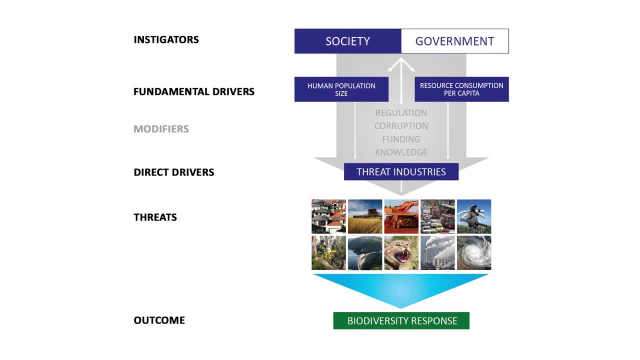 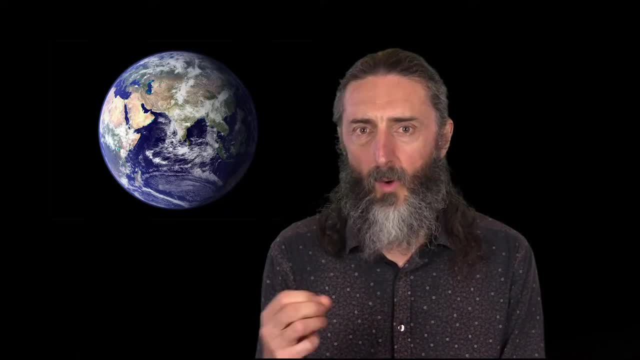 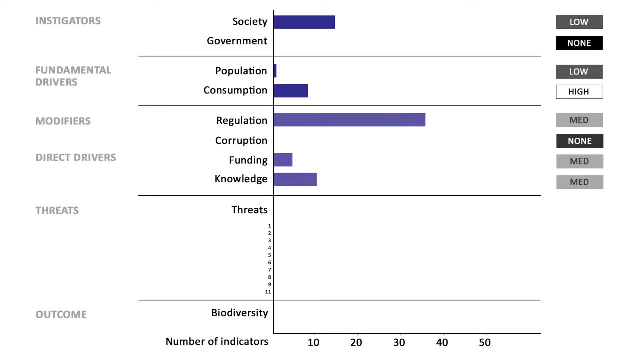 The combined actions of society and government can modify the impact of threat industries through regulation, corruption, funding for the environment and knowledge about biodiversity. So how well do indicators represent the components of the biodiversity crisis hierarchy? A count of the number of indicators reveals some startling gaps, Even though government 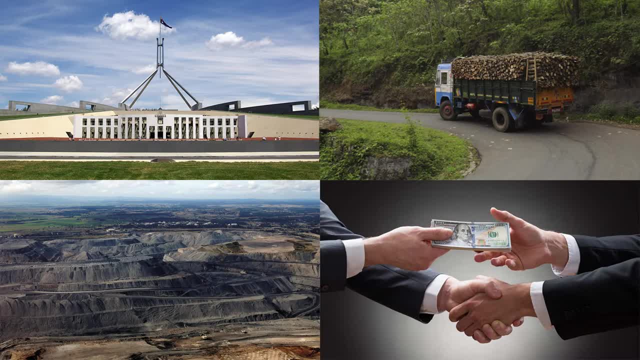 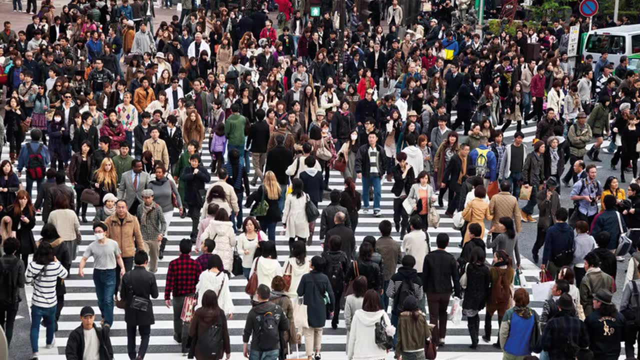 corruption, mining and roads have enormous influence on biodiversity. they had no evidence of the impact of the crisis And, while human population size is a fundamental driver of the biodiversity crisis, there is only one indicator related to that. Another way to evaluate how well indicators represent the hierarchy is to look at the 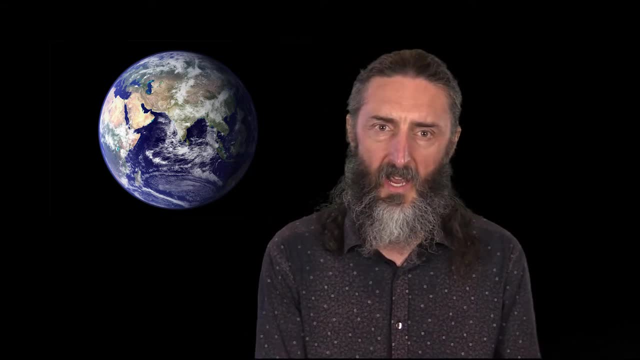 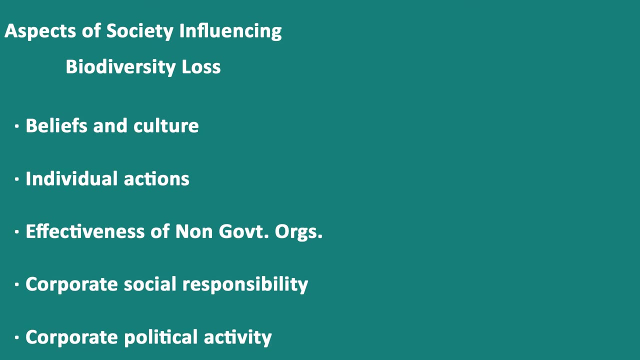 scope of each component of the hierarchy relative to the scope of the indicators. For example, the aspects of society that influence biodiversity loss includes beliefs and culture, individual actions, effectiveness of NGOs and corporate social responsibility and corporate political activity. There are 16 indicators for society. Ten were about measuring benefits from nature. one